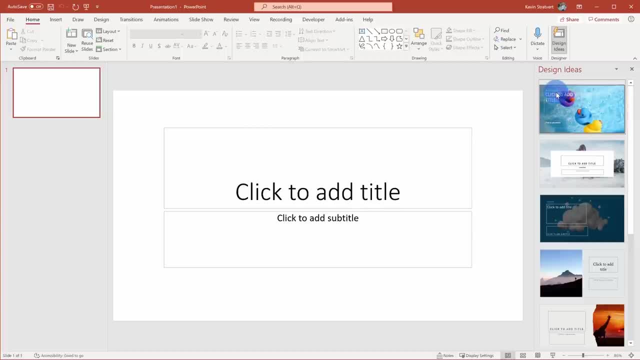 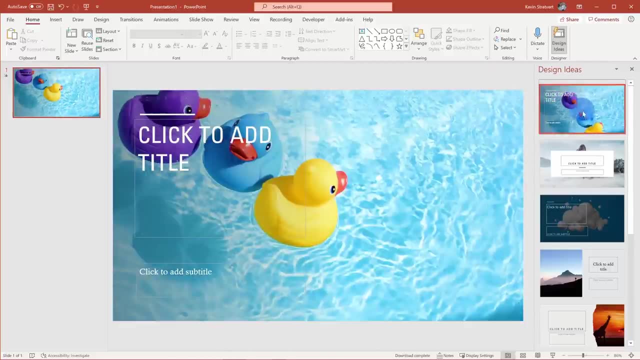 the first one has a video background. so design ideas now also includes video. Here I can click on this and this will insert it directly into my presentation. so now I have a video background. Now you'll notice there's only one video background here out of this set. 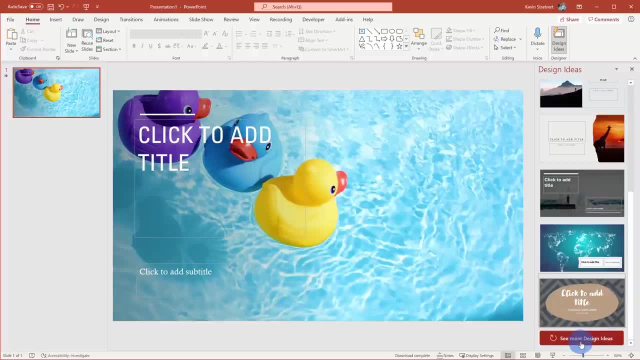 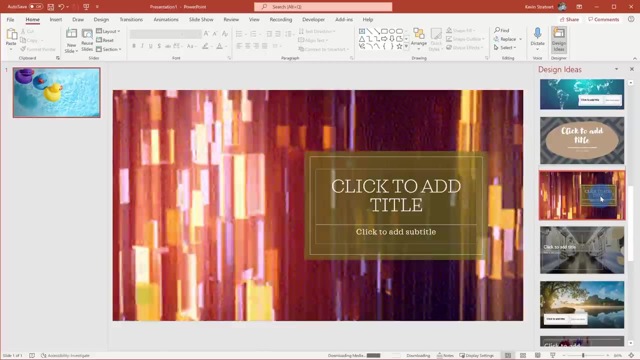 Now you'll notice there's only one video background here out of this set, But if I go all the way to the bottom of this design ideas pane, I could also click on this see more design ideas, and when I do that it'll show me even more options. and here's another one with a video. 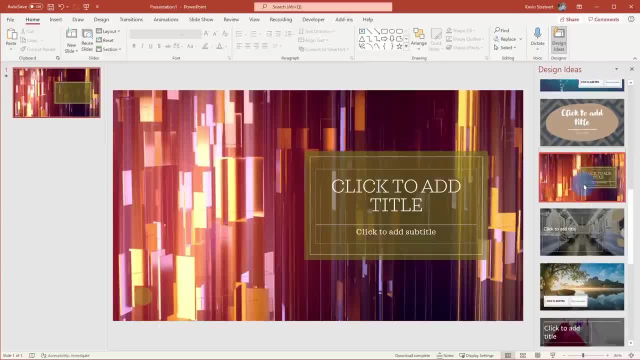 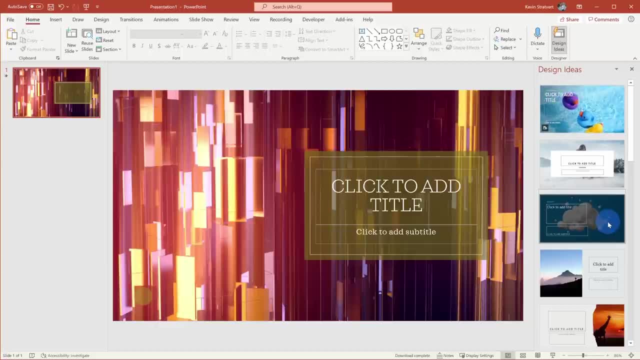 background and I can click on that and simply insert that into my slide as well. Design ideas is a really nice way to create a presentation very quickly and also to make sure that it looks very good Now that I've added my video background to the slide. 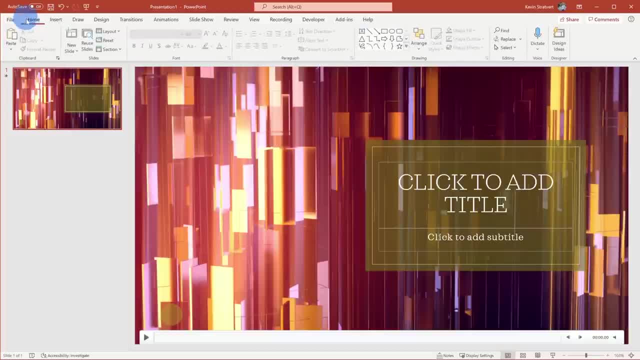 I can add content on top of it. Here you'll see that this is currently set to a title slide, so here I could come in and let me add my name to the title slide, Along with simply typing in text here. maybe I want to paste an image I'll put in the 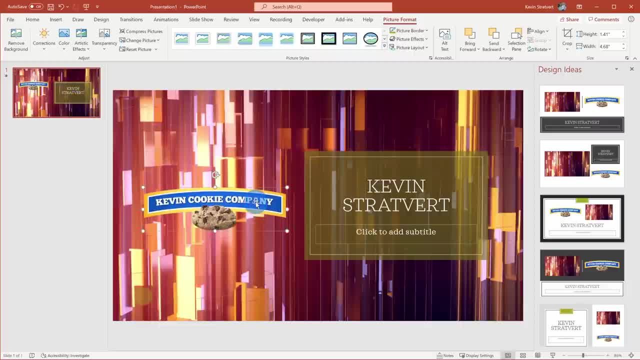 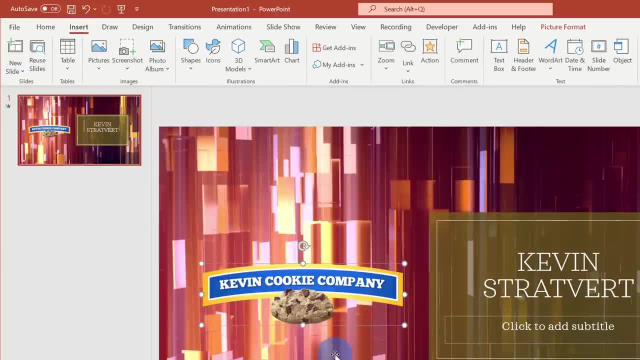 logo of the Kevin Cookie Company and I'll position that right over there. In fact, I can go up to the insert tab and I can insert any type of content on top of this video background. Now that I've added a few things, let's jump into presentation mode to. 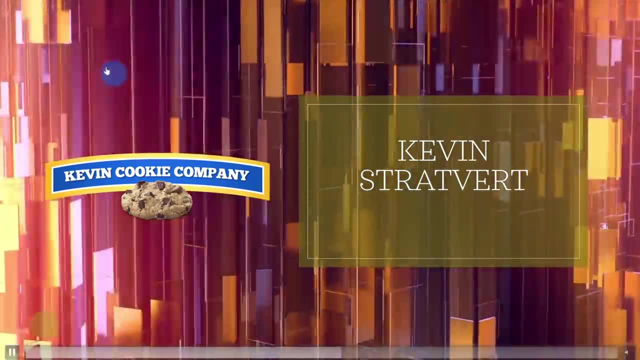 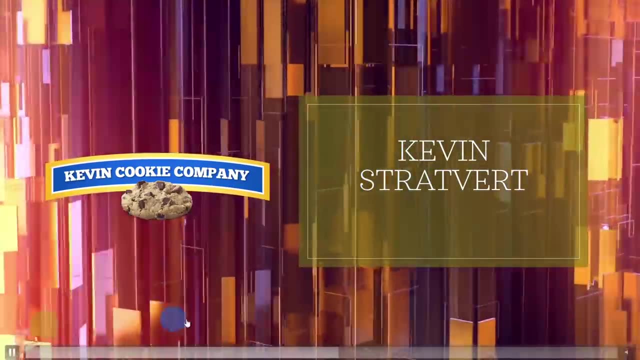 see what this looks like Here within slideshow mode. some of the things you'll notice. is it just automatically? Also, as the video plays, it automatically loops. So once it reaches the end, it'll just keep playing again and again. And the good thing is the way the video was designed is. 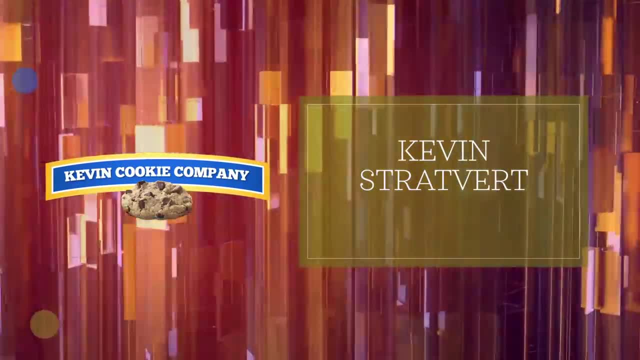 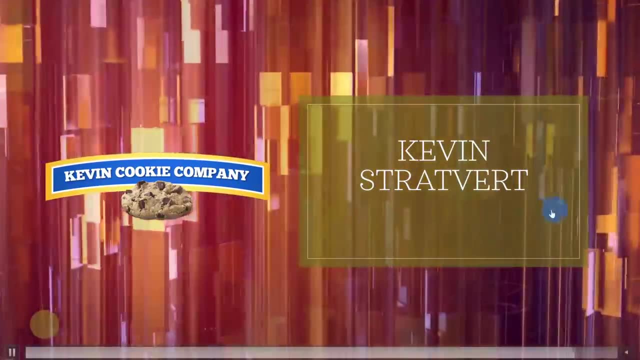 it's not really noticeable that the video is looping. It just looks like one continuous long play, and that tends to work really well for a video background. Another thing that really impresses me if we look at the text here. look at that transparency. So the video continues to. 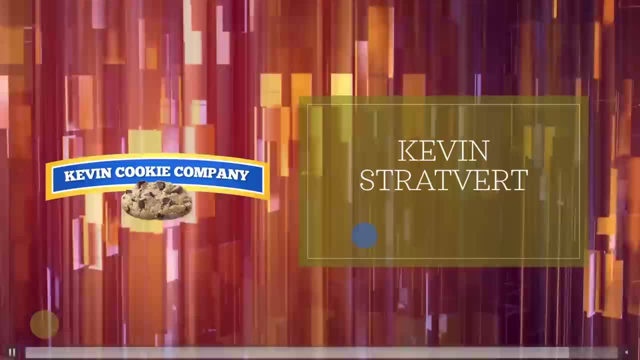 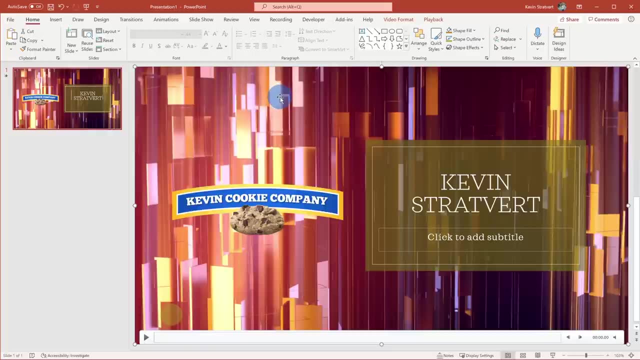 play in back of this object. So overall, this looks really nice. Back now on the main screen, I can select the video background. This is my currently selected object, And when I select this, you'll see that there's a new tab up on top called playback. When I click on this one, 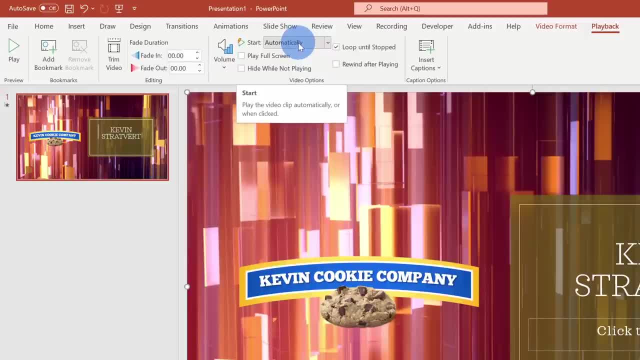 right in the center I have video options, And here I can confirm that the video will just automatically start playing and it'll continue looping until stopped. Now I would recommend leaving these settings. This works extremely well for a video background, Now that we've 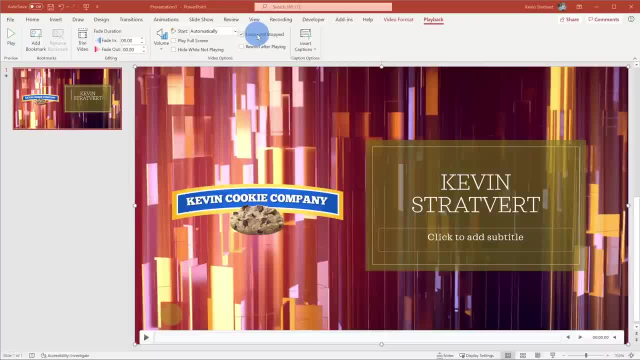 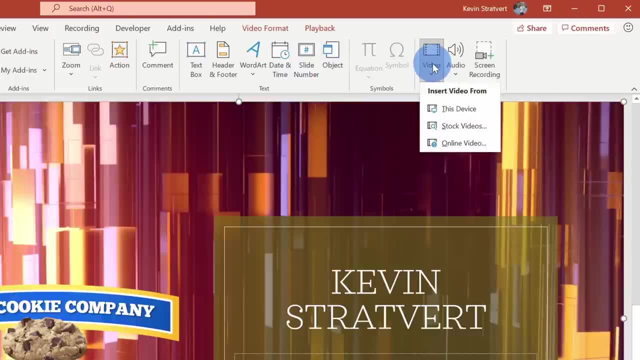 looked at these settings. let's see how we can access even more video backgrounds. In the top tabs, go over to the one that says insert and all the way over on the right-hand side you'll see an option to insert videos And within this menu there's the option for. 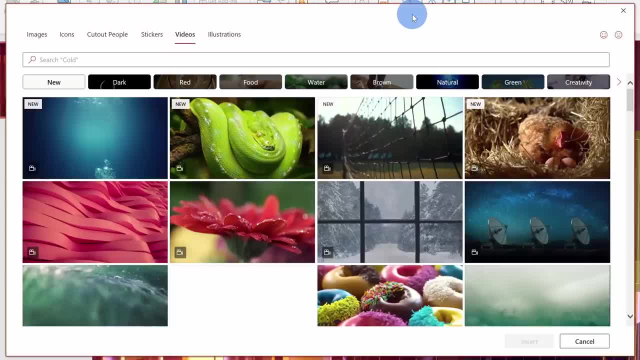 stock videos. Let's click on that one. This opens up a prompt with stock videos, and here you have a massive collection of different videos that you can insert into your presentation, And along with videos there are all sorts of other stock content that you. 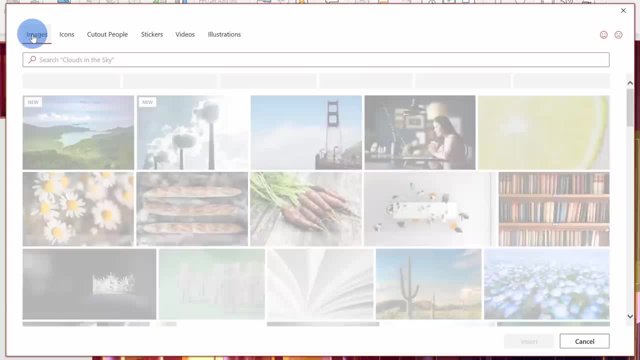 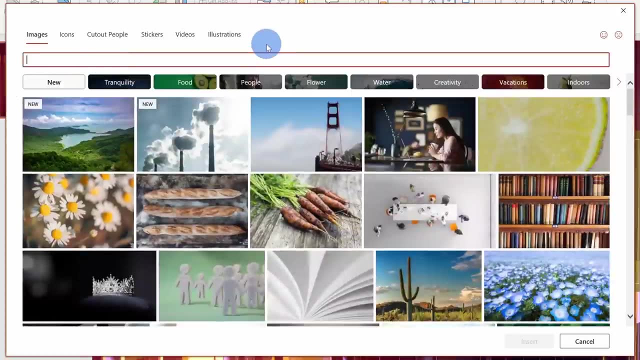 can also insert into your presentations. For instance, over here on the left-hand side you can insert different images And here you have a ton of images to choose from. You could even search for images. So let's say, I want images that are red Here. I'll type in red and look at that. It gives me back all these. 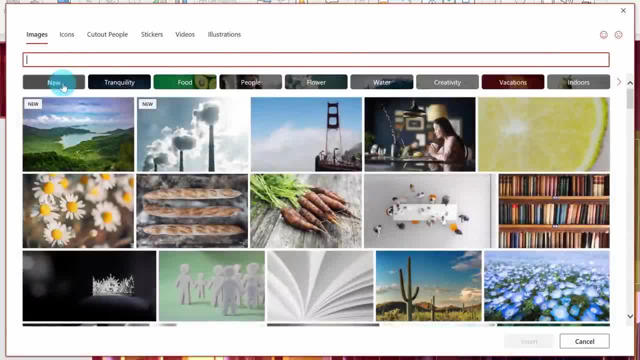 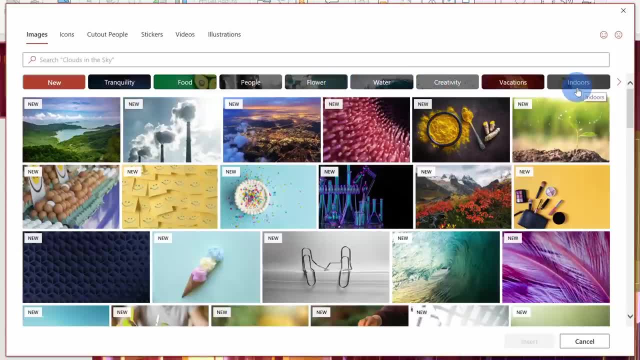 different red images Here, I'll cancel out the query. I could also look at all the new images that were added, or I could choose from one of these categories, So it's really easy to get to the type of content that you're looking for Up on top. I could also insert icons into my 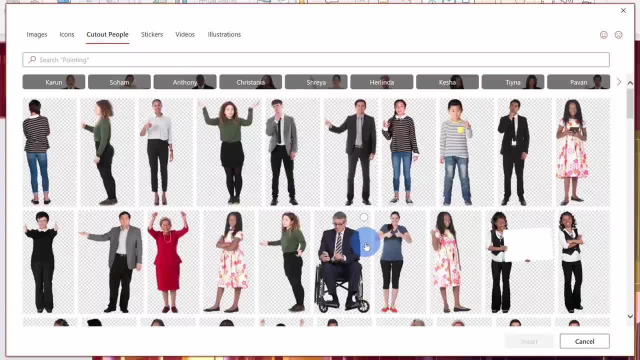 presentation, I could insert cutout people. Now, the cutout people are really cool. You'll notice this grid background in back of them. This is a transparent background, So if you insert one of these images, it's really easy to integrate it into your slide. To the right: of cutout people. 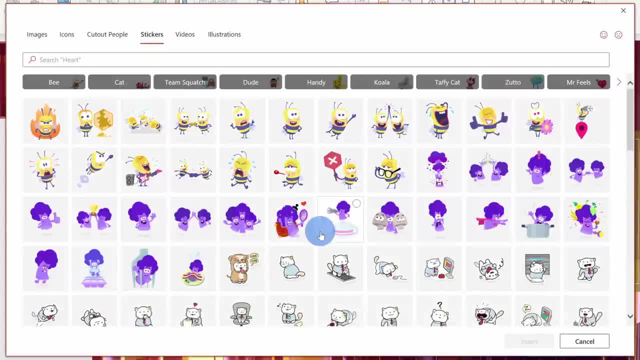 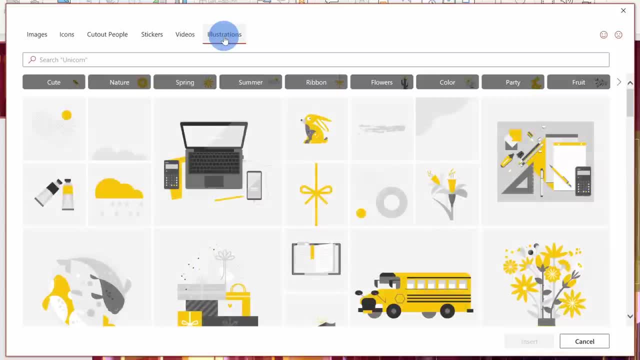 I can also insert stickers. Maybe you're a teacher and you're reviewing a student's presentation. You could insert one of these stickers in And all the way over on the right hand side you also have stock illustrations that you can insert, And here too, just like all the 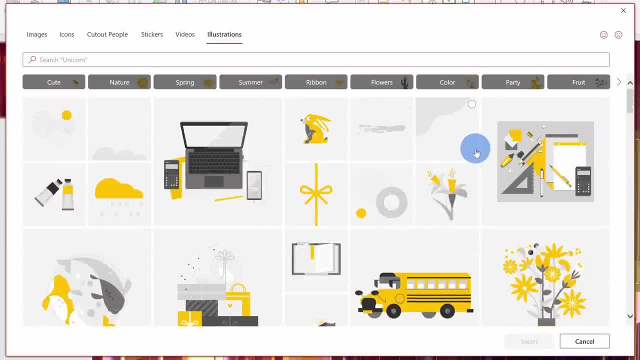 other ones. you have many different options. One of the neat things about illustrations: you'll see yellow incorporated into them. You can change this color once you insert the illustration. All right, let's jump back into videos and see what we could do here. So look at all of these. 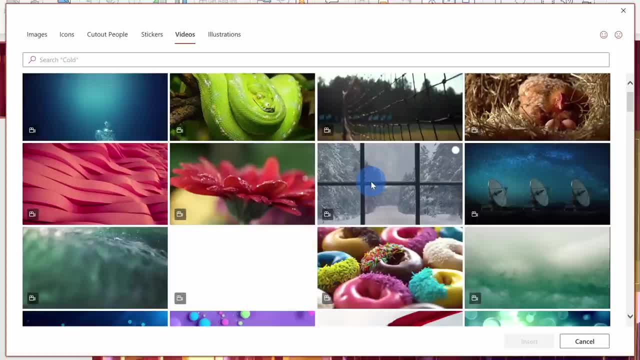 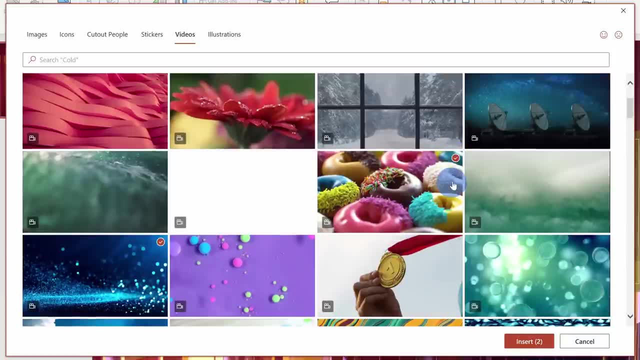 different options Here. if I hover over I could get a preview of what that video looks like. Here I'll select one of these videos. Maybe I'll go through and select another one And here you'll notice you could select multiple videos to insert into your presentation. I'll pick these three. 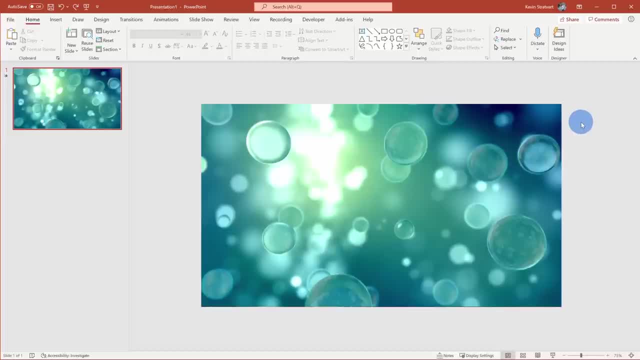 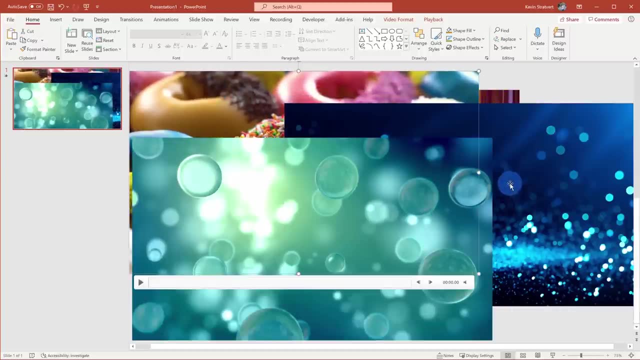 and then I'll click on insert. I've now inserted my three video backgrounds And just to confirm that there are three backgrounds here, I'm going to click on insert And I'm going to click on insert Here I can move them just a little bit and you can see all of these different video. 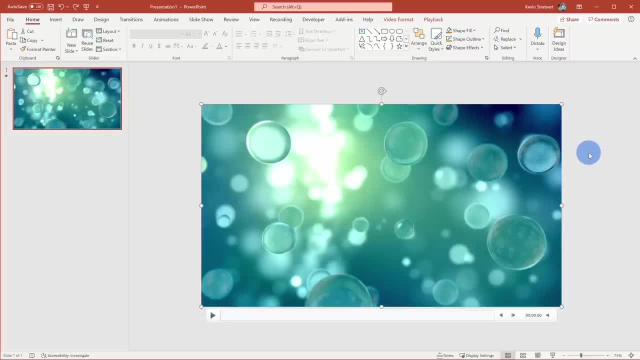 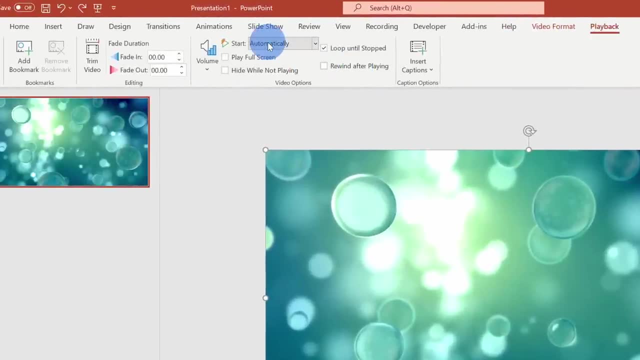 backgrounds. I'll undo that, so they all just land in a stack again Here. when I select the topmost video, if I click on the playback tab on top, here too you'll see that it's automatically set to just start playing and then also to loop until stopped, So it has the same settings as the. 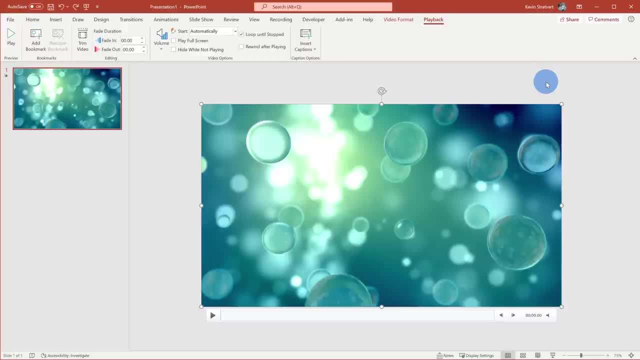 original video background that we inserted. Now let's say that I want to evaluate which video background looks the best with my content. I can use the selection pane to help me with this. Here I'll go over to the home tab up on top and all the way over on the right. 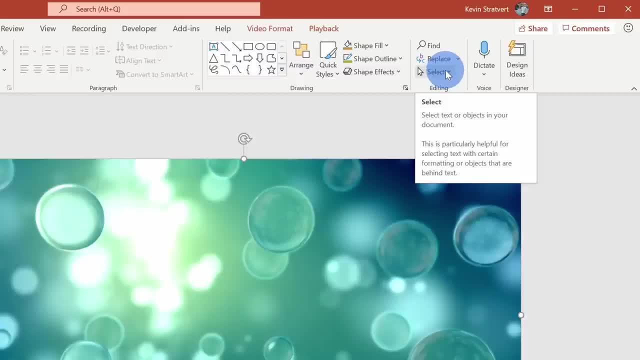 hand side, there's the option that says select. If you've never used this before, this is super helpful, as you're organizing different shapes on your slides Here. I'll click on this and I'll select the selection pane Now as a quick shortcut key. this is one that I recently learned about and 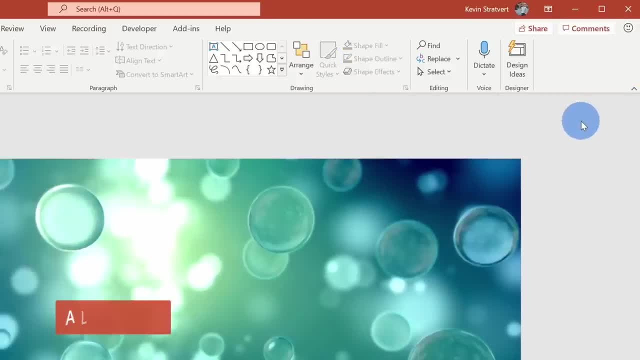 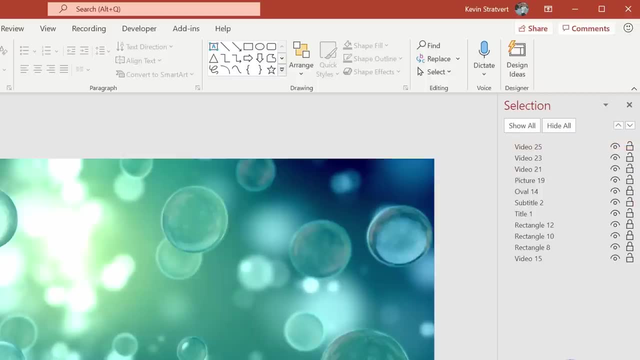 it is extremely helpful Here. I'll close the selection pane. You can press the alt key together and it will take you to the selection pane, So very quick way to get back to this. Within the selection pane, whatever item is at the top is the topmost layer, and whatever item is at the bottom 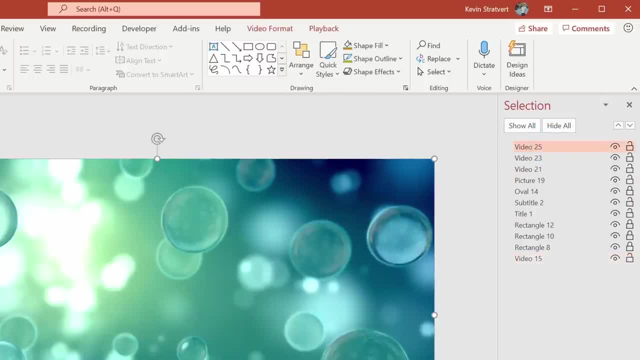 is the bottom most layer Here. if I select video 25, I'll see that it's this video with the bubbles, and if I click on video 15,, well, this is the original video that I added. We can't see it because it's behind everything else right now. Now, let's say I want to evaluate these different. 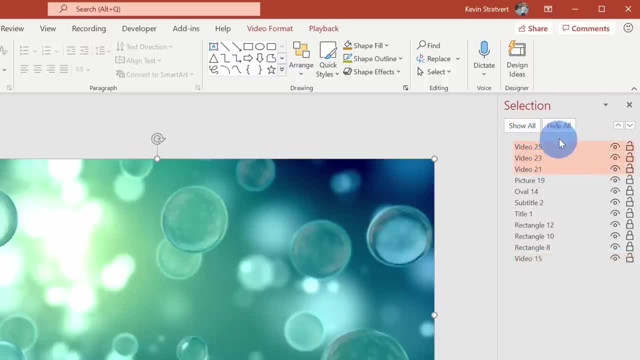 video backgrounds in back of my content. I'll press the control key so I could select all three of them and I'll simply drag it underneath all of this other content, but I'll put it ahead of video 15, which is the original video. 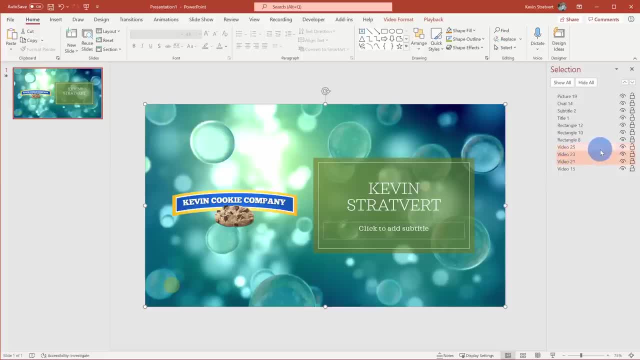 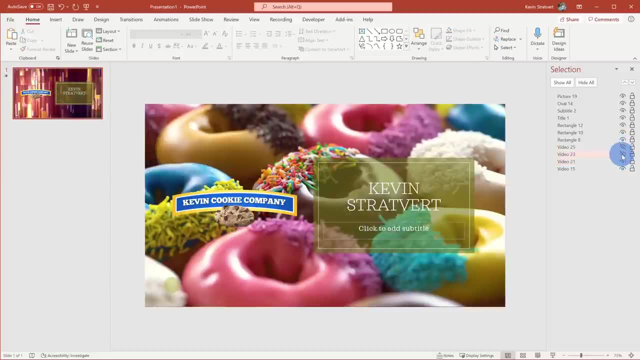 So I'll place them there and here. now I could evaluate what they look like, So I could go through each one and I could click on this show or hide icon and so I could hide that and I can view the next background, and here I could go through and decide which one I like the most. 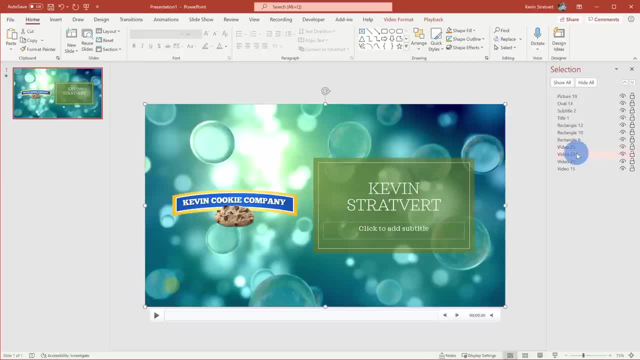 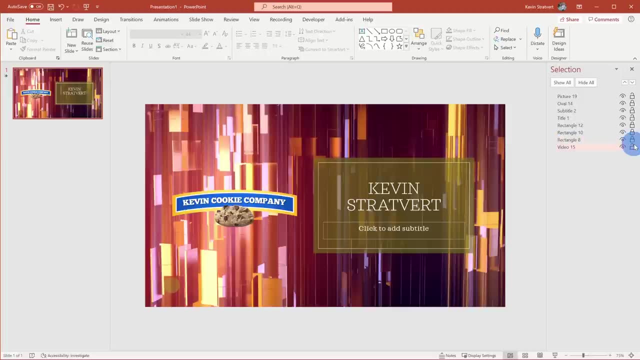 Now I personally think the original one looks the best. so here I'll select the three video backgrounds that I added. I'll press the control key once again, highlight these three and I'll press the delete key to remove those different selections. and here I am back to my original video background. I thought this one looked pretty good. 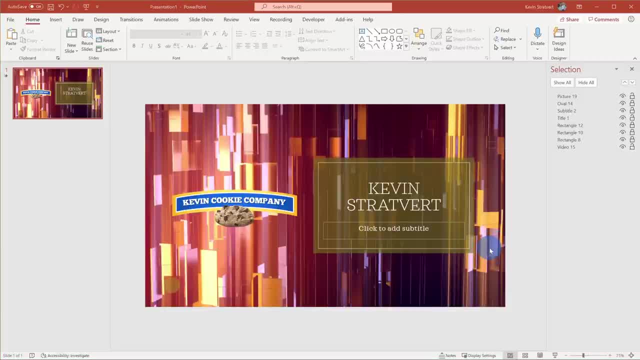 Let's say that you want to use this video background somewhere else. Maybe you want to use it outside of PowerPoint. Well, you could very easily do that Here. once again, I'll select the video background and you can right click on it and then go down to save media as. 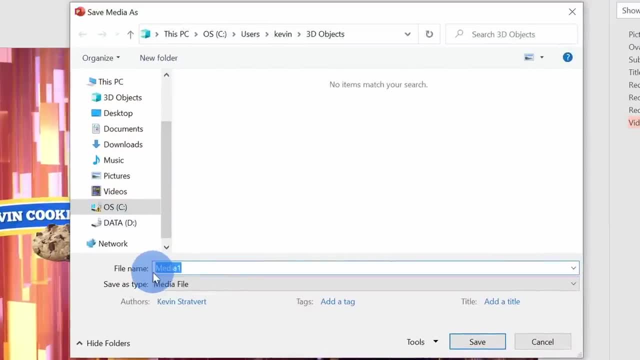 When I click on that, that'll open up the windows save as dialog. Here I could type in a name for this video clip And it'll save it as an mp4.. Once I'm done with that, I can then click on save. 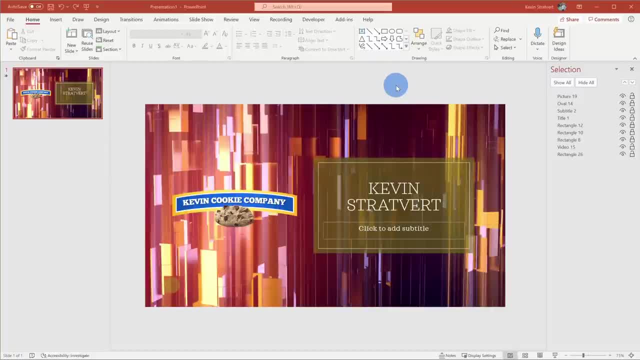 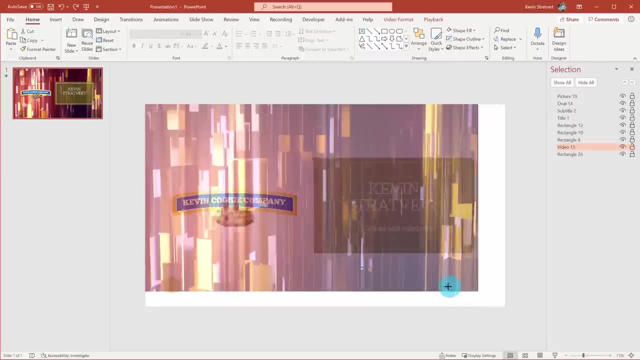 Back now on the main screen. I want to show you some other things that you can do with these video backgrounds Now. right now, the background is set, so it uses up the entire slide. However, I can resize this, So maybe I just want a video background behind. 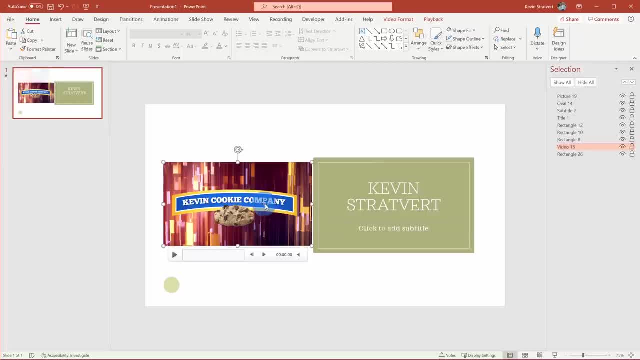 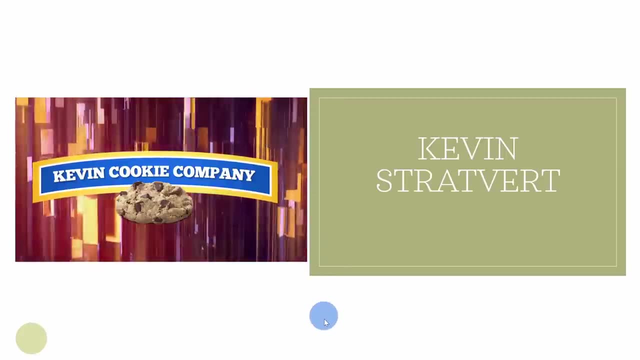 one of the elements on the slide, So maybe I'll just place it behind the logo right here. When I launch into presentation mode here, you'll see that the background plays just like it did before. but now, in this specific area, I'm going to resize it. But when I click on the video clip and go up to the top tabs, 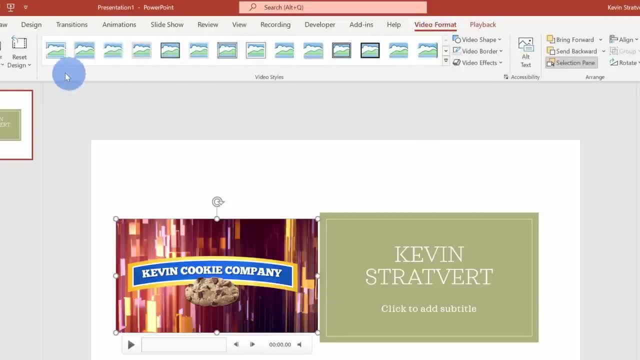 I can click on video format And here I can select from all of these different formatting options. Over here I could apply a video shape. When I click on this, I don't know, maybe I go with this banner down here and that'll adjust it to a banner Right up here I could also apply different. 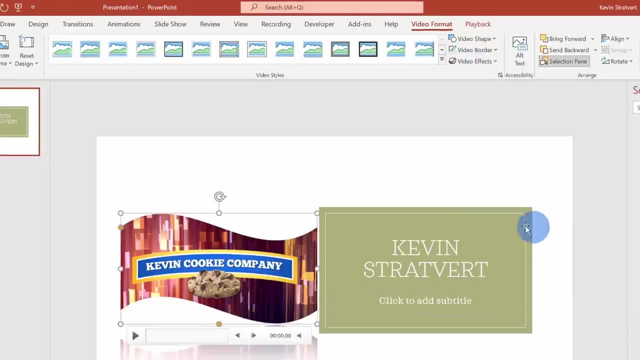 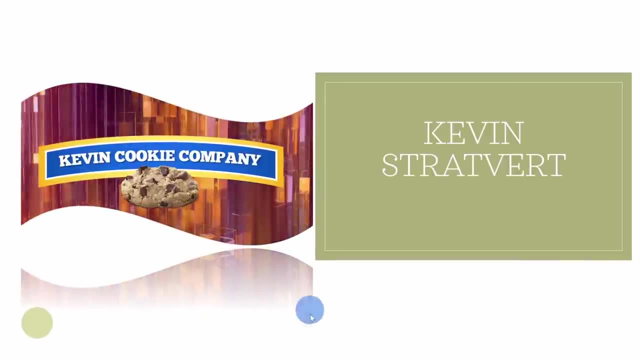 video effects. So maybe I'll add a, let's say, a reflection. I'll throw in a reflection and let's once again jump into presentation mode And look at that, It now applies that shape to my video and unless it applies a reflection, and look at that, the reflection also plays the video. 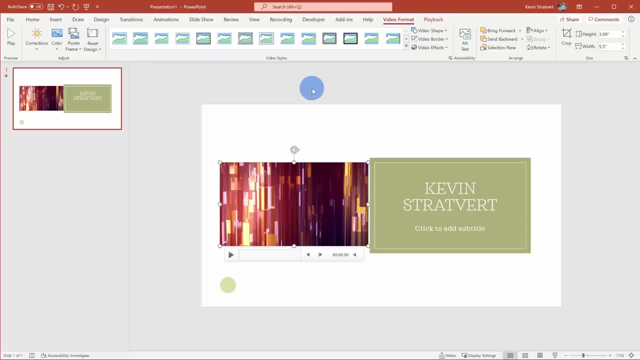 So you could do some really fancy looking things. Lastly- and this is a good one- I want to show you how you can play your video in a custom shape. Here, once again, I have the video selected, and previously we went to video format and we applied a video. 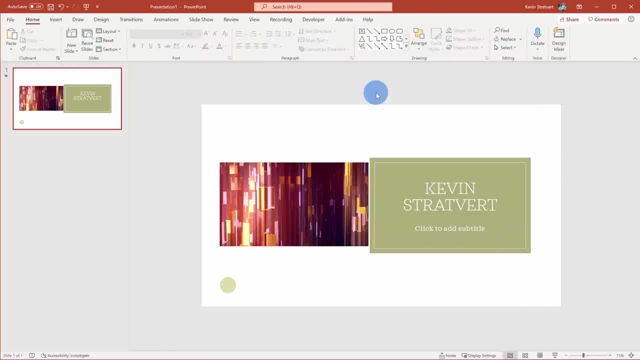 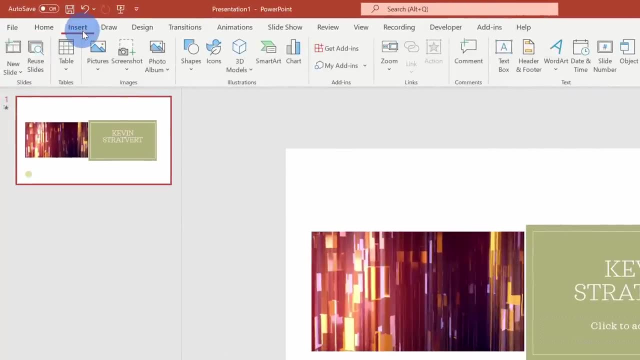 shape to this video. But next I want to show you how we can play the video in- I don't know, maybe a cookie Here. I'll go up to the insert tab up on top And earlier to get to the stock video. I clicked on video and I selected stock videos. 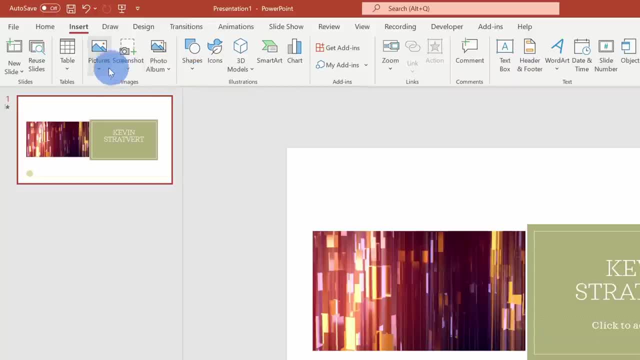 but there are many other entry points. Let's say, I want to insert a stock image, Here I'll click on pictures and I could select stock images. Or if I want to select a stock icon, here I could click on stock icons. So once again, many different ways in. I'll click on stock icons and let me 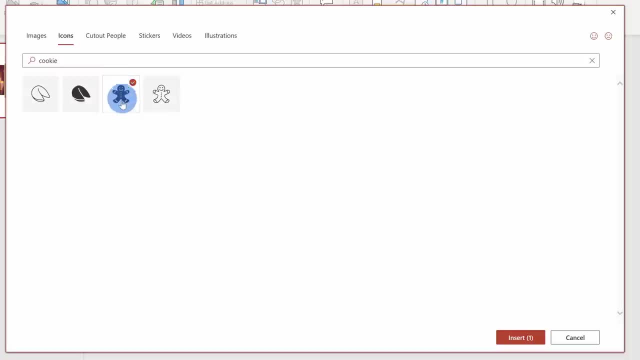 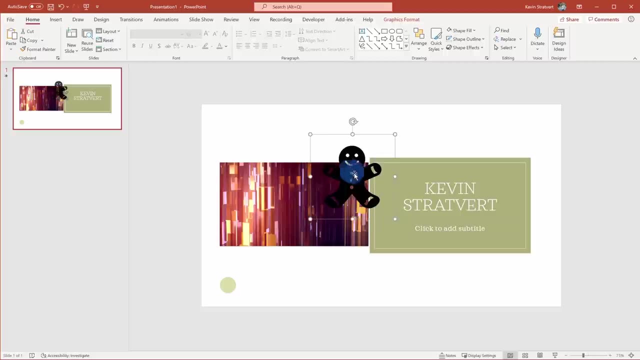 search for cookie. Here's a nice picture of a gingerbread cookie. I'll select that and then click on insert. I've now inserted my gingerbread man and here I'll resize him so he's a little bit smaller, And I'll place him in front of this video. Next, I need to convert this from a vector. 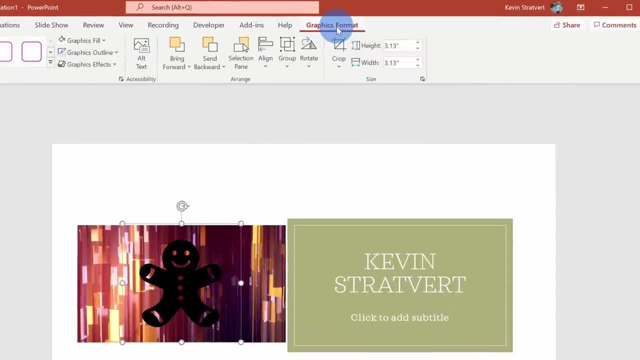 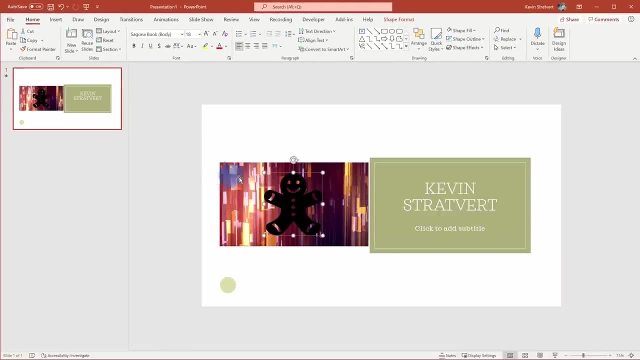 image to a shape. I'll select the gingerbread man and go to graphics format Over on the left-hand side. here I can convert to a shape. I'll click on that. So now it's just a standard shape. Next I'll select the video, and you want to make sure you select the video first. Then press the. 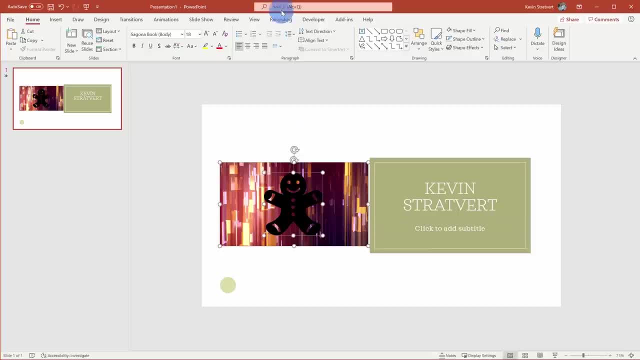 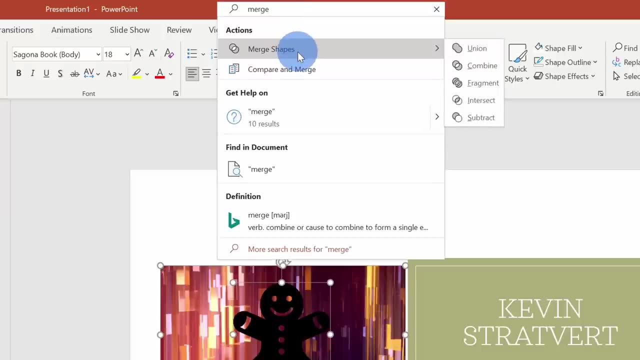 control key and select your object on top. In my case it's the gingerbread man Right up here. in the search field I'll type in merge. I'm going to use the option to merge shapes, So we're going to merge this shape with the video. 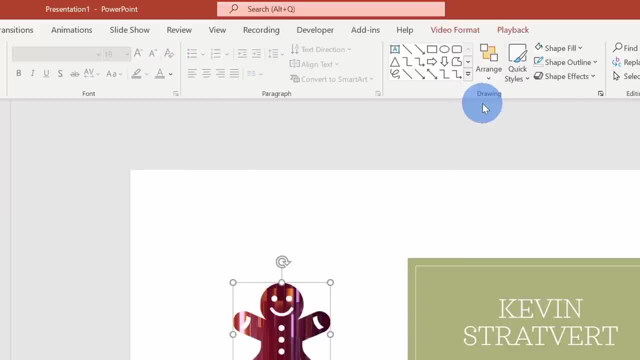 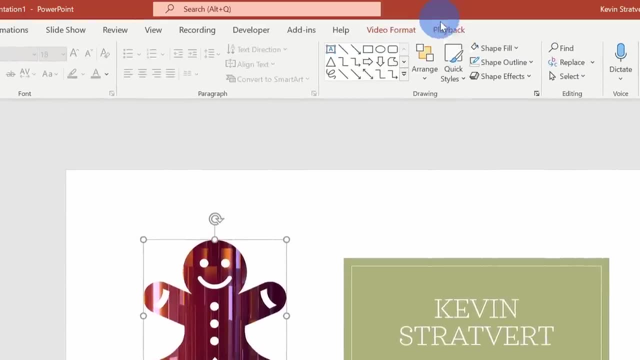 And we have different options, but we want to select the one called intersect And when I select that, look at that The video now fills up- the gingerbread man. With the gingerbread man selected, go up to the top tabs and click on playback And over here, let's set it to start automatically. 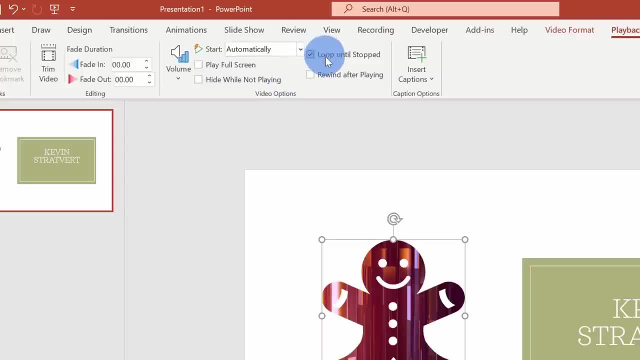 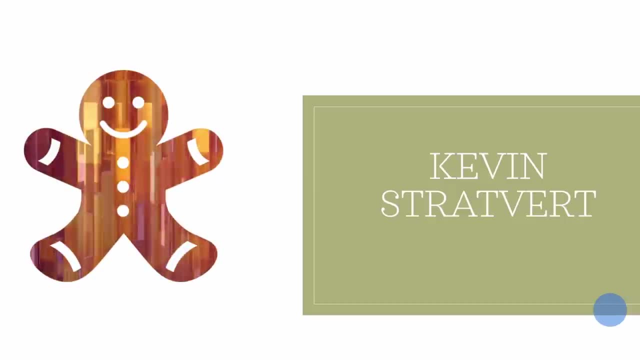 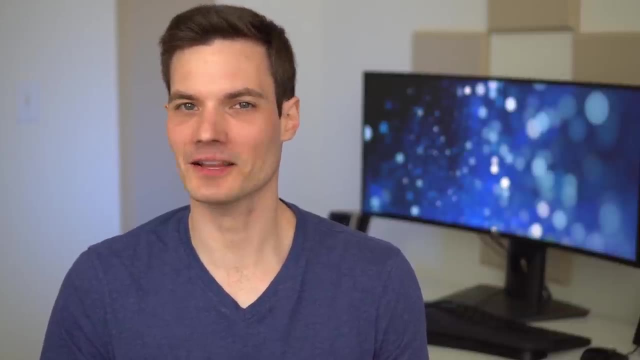 And let's also loop until stopped. With those options configured, let's go down and play the slideshow And check out that Our video now plays within the shape. These tips are sure to impress whoever you're presenting to All right, Well, that's how easy it is to insert a video background. Let me know down below in the 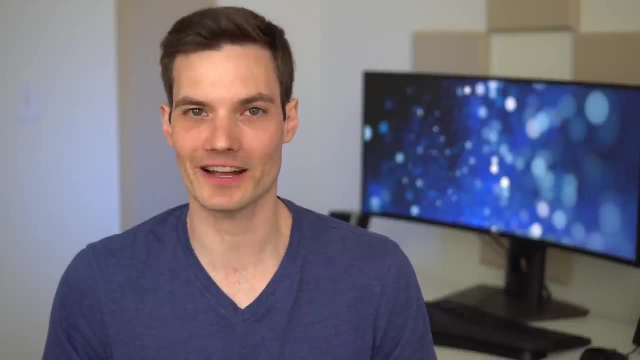 comments. Are you planning on using this And maybe, if you did already, what was the reaction of your audience? If you enjoyed this video, please consider subscribing. All right, Well, that's all I have for you today. I hope you enjoyed And, as always, I hope to see you next. time Bye, Bye.